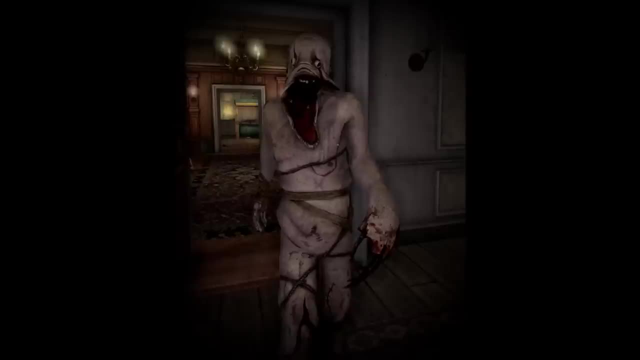 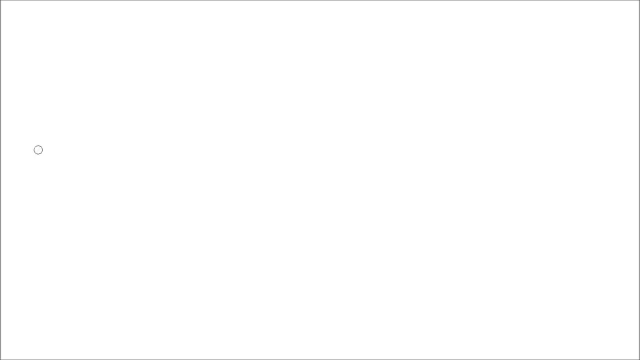 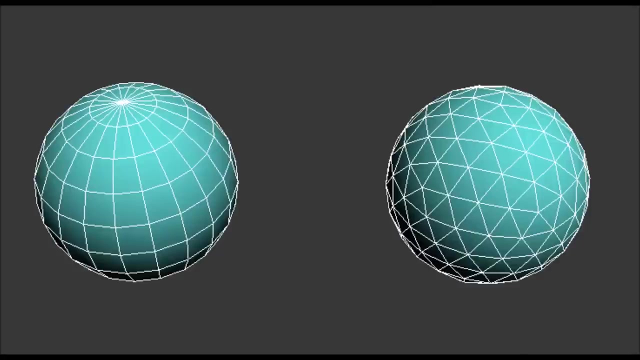 How do graphics go from zeros and ones to characters on your screen? Well, let's learn how graphics work. First things first. all 3D models are made up of triangles or squares, also called quads. Now, these shapes may look simple, but they can be used to make 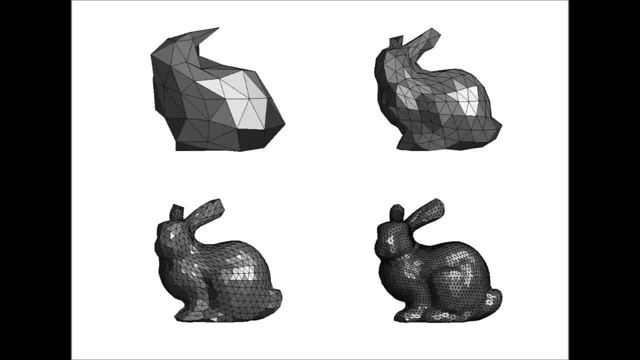 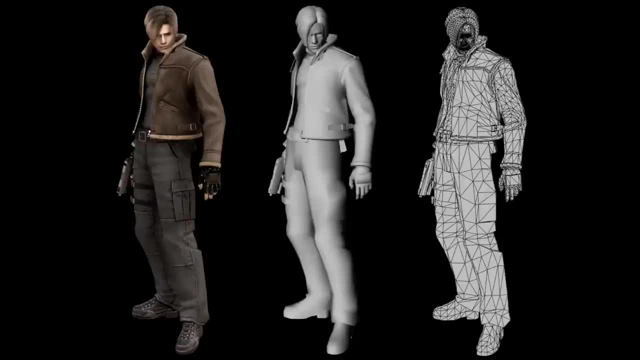 pretty much anything you can imagine, And the more shapes you have, the more detailed your object becomes. Now there's different costs and benefits to using one or the other, but all of your favorite characters are made up of one of the two. First, let's draw some shapes. 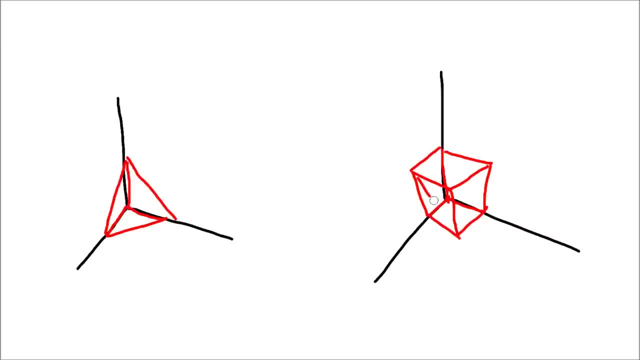 using triangles, We can call these models, And we're using 3D coordinates to define these models, which is just a way to keep track of what the shapes look like, so we can easily send that information to a computer. Now notice that there's an x, y and z axis, which basically just 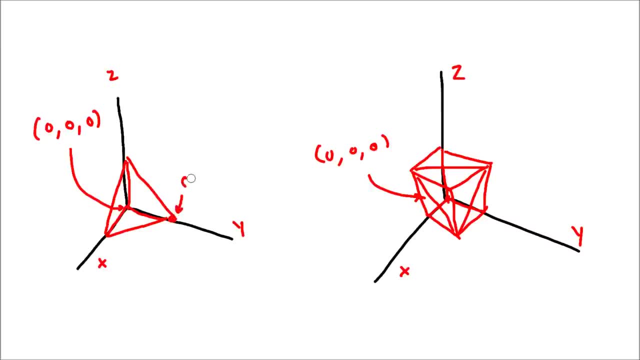 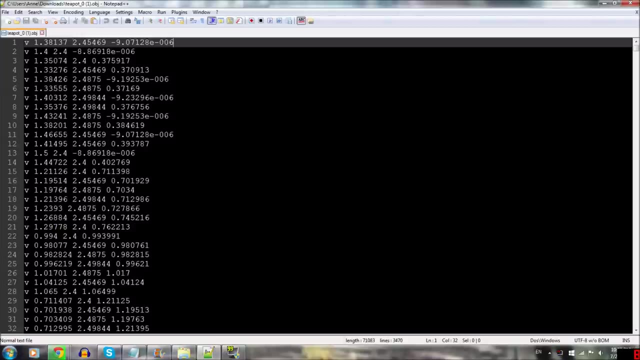 means length, width and height, And notice that all of these shapes have many varying points along the edges, but they could be defined by four in the case of a square, So we can call these shapes in the case of the model on the left, and those four points are called the vertices. This is a file. 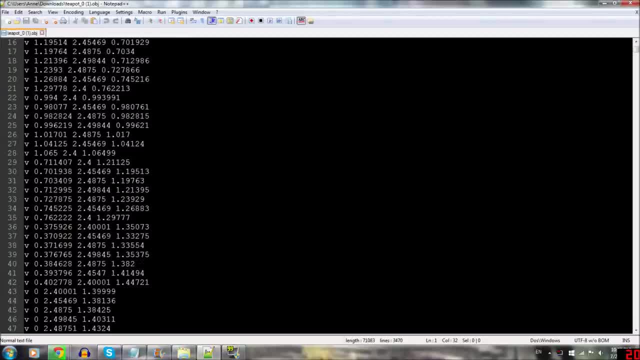 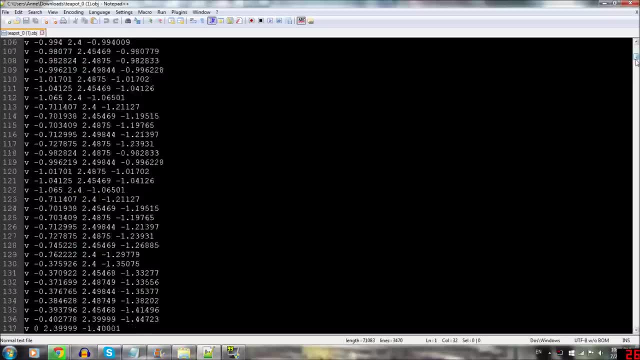 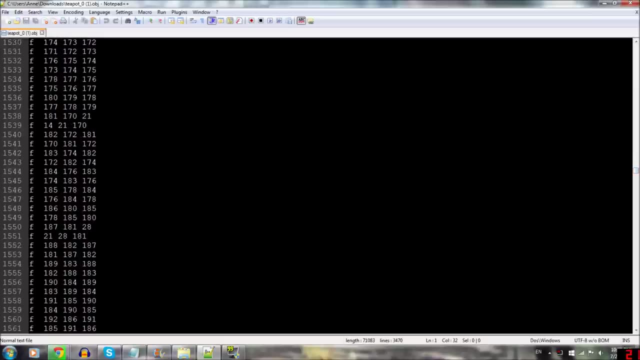 of a fairly complex 3D model, broken down to its barest bones. The v's represent the vertices followed by the x, y and z coordinate of the point or vertex that defines the shape. Moving down we have the faces. where f123 means draw a triangle using vertex 1,, 2, and 3 from the list above. 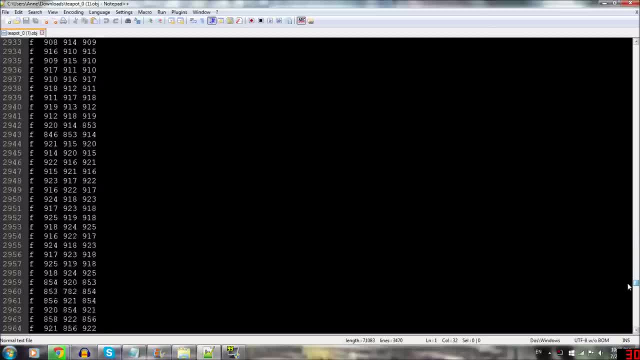 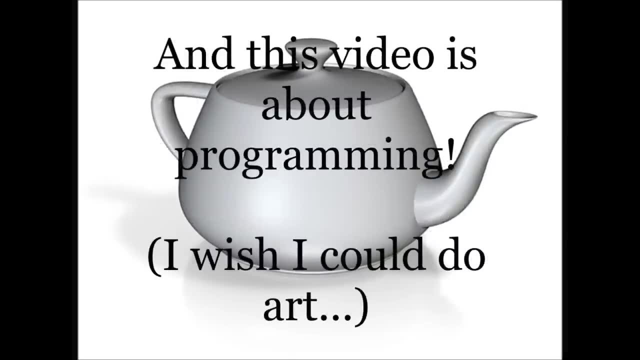 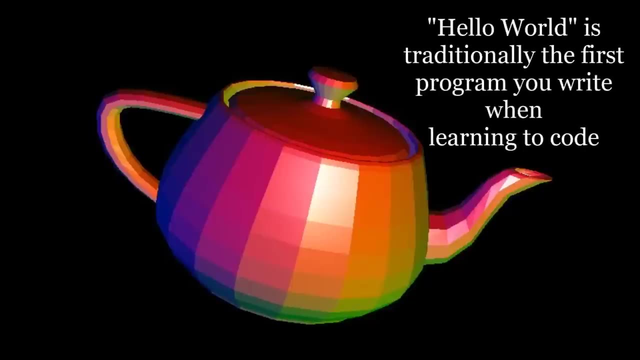 This is a good time to note that graphics artists are not just sitting there typing in points until you get something that looks like this, which is what the file was defining. by the way, This may sound weird, but people in graphics love teapots. They're kind of the hello world of OpenGL and the 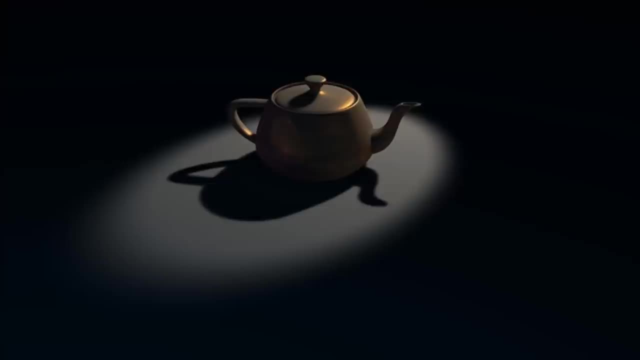 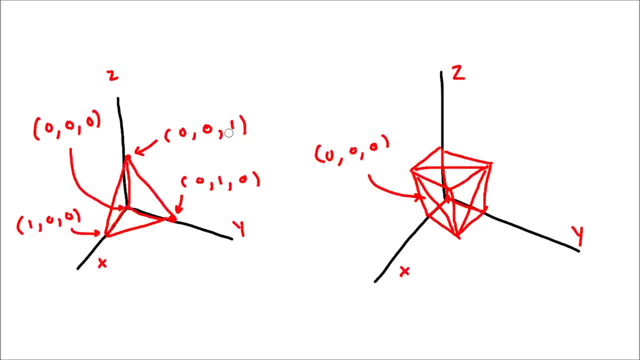 graphics world, And they're complex curved objects that are pretty good for trying out new texturing or lighting techniques. Anyway, let's look back to our models from before. This is how they both start at, also known as the origin. Now, if this is a game world, 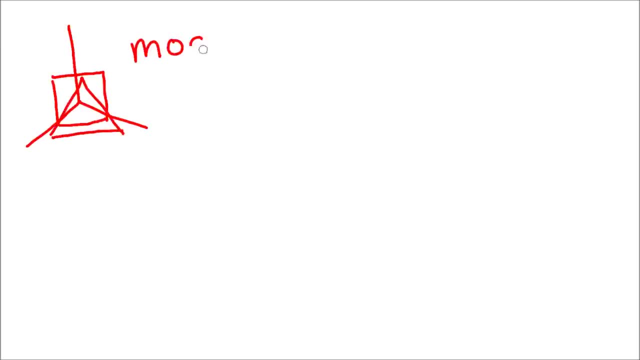 you can't have everything starting at the same spot right. Everything would overlap. This is why we have to keep track of different coordinate systems. In this case there are world coordinates and model coordinates. We can transform the model's coordinates to the world. 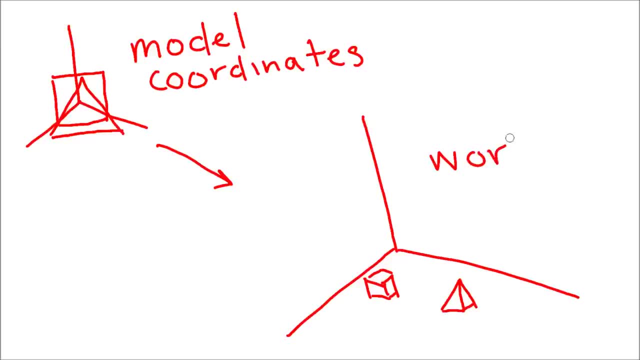 by multiplying matrices. Just know that a matrix is like a grid where we can store all these coordinates and we can store all the coordinates that we want to store in the world And we can multiply different grids to go between different coordinate systems. The example below shows how 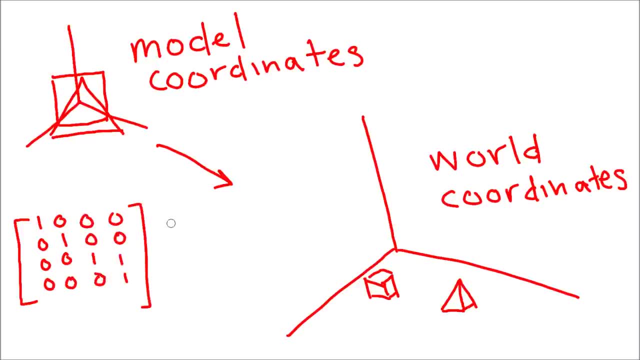 you'd use matrices to shift a model one unit up, as an example. This way, we can separate how we keep track of the object's shape from how we keep track of where it is in the world. Now that we've placed our models in the world, we have to think about how we want to view them. 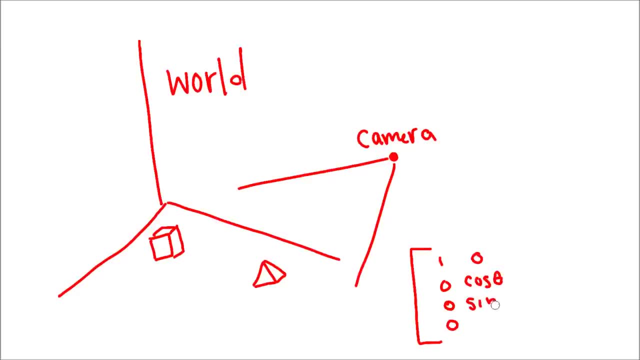 and create the camera. Once again, we use matrices to rotate our view. However, we now have to two options. We can either rotate the camera relative to the world or the world relative to the camera. In other words, we could move the camera around like you might in real life. 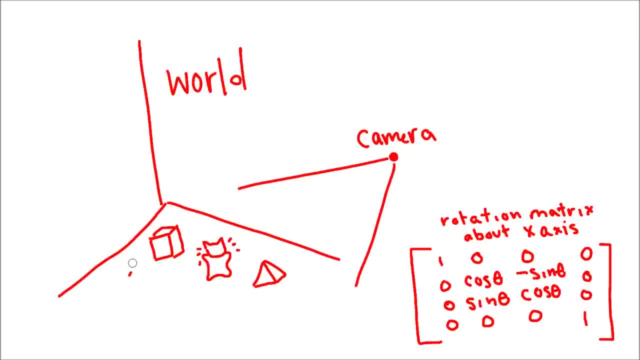 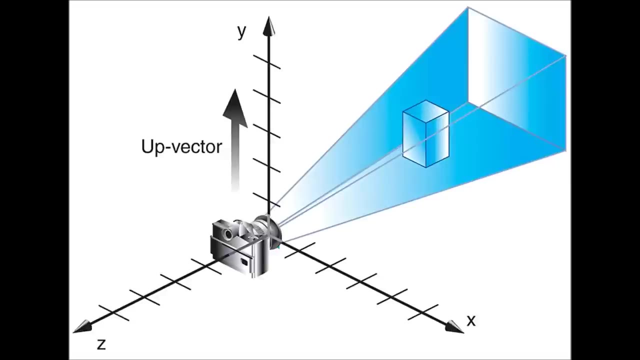 or we could keep the camera in one place and have the entire world move around that point, While the second one seems way more difficult to imagine. that's actually how graphics work in practice. This is because the idea of a camera is an analogy. There is no camera. 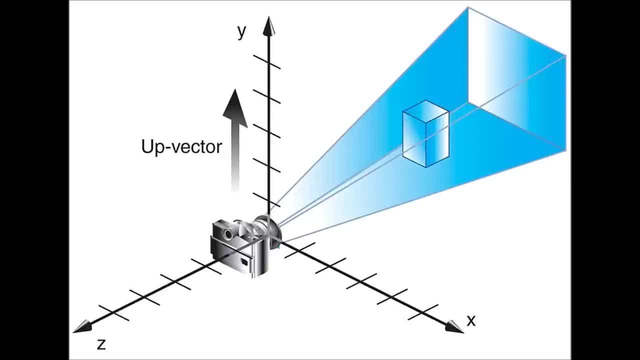 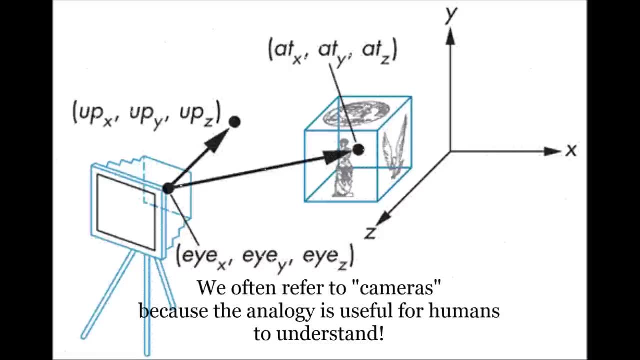 Your window is a view into the game world and the programmer tells it what to display. Adding a fixed point and calling it a camera actually would require more math and it slows things down a bit. So we have coordinates representing models, models in our world. 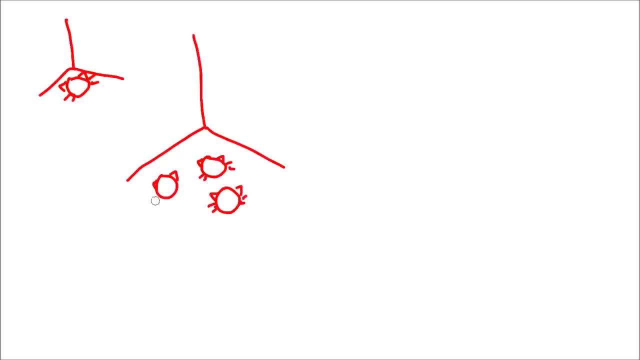 and a camera to move around and examine things with. Now we have to make all of that display on a screen. Something people don't often think about is that 3D games aren't actually 3D. Your screen is obviously flat and each tiny pixel displays exactly one color In games.